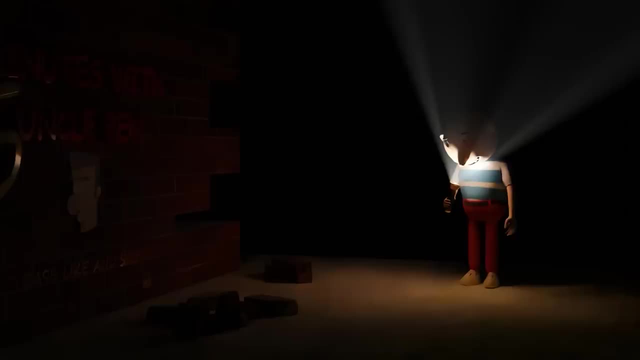 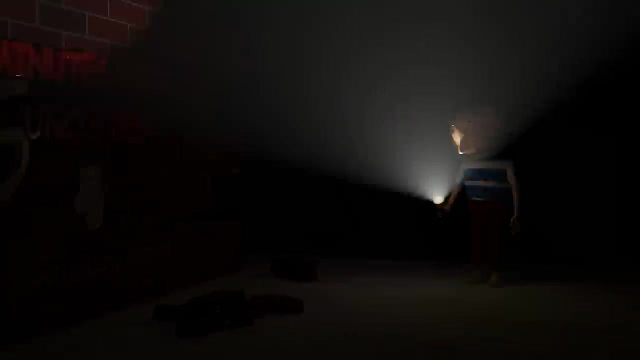 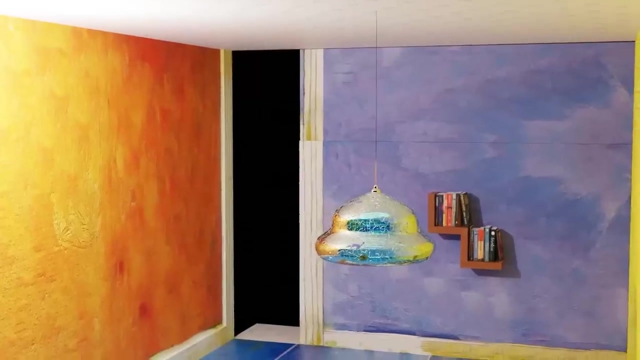 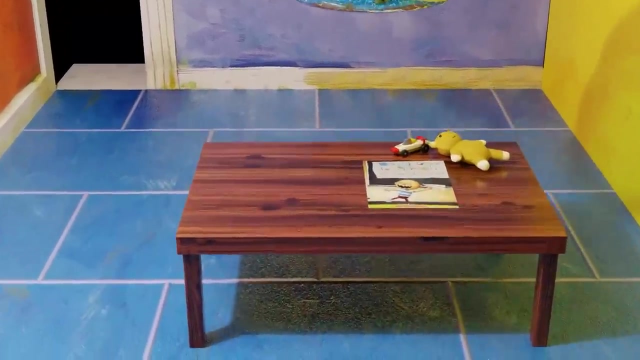 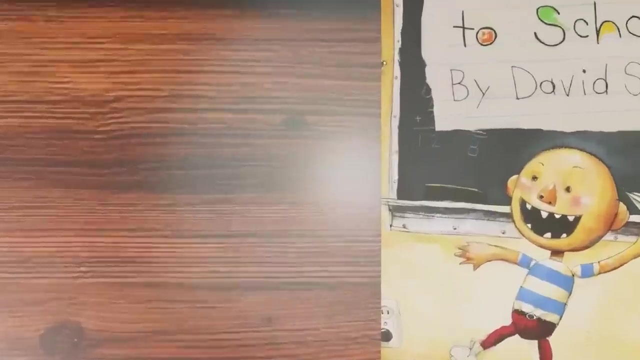 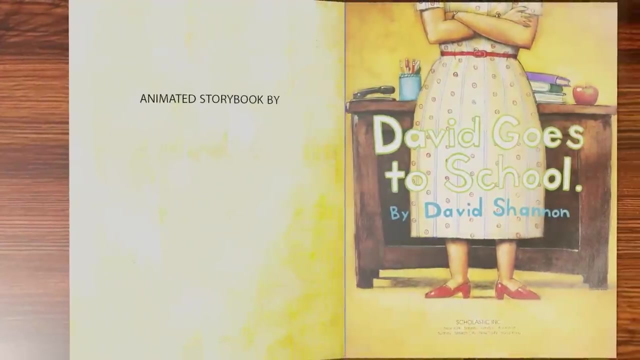 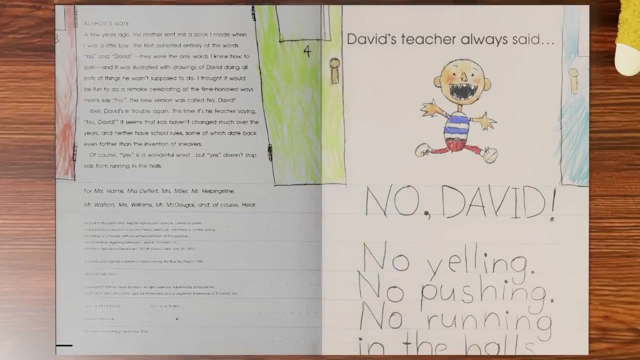 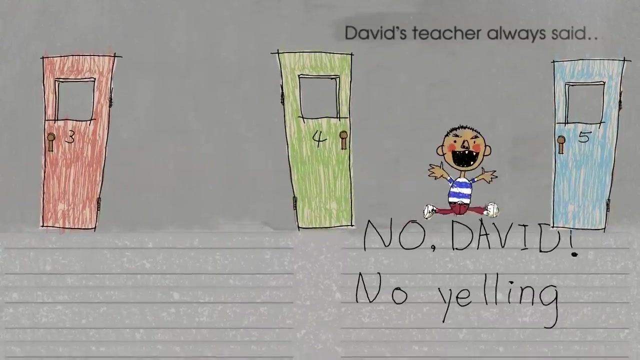 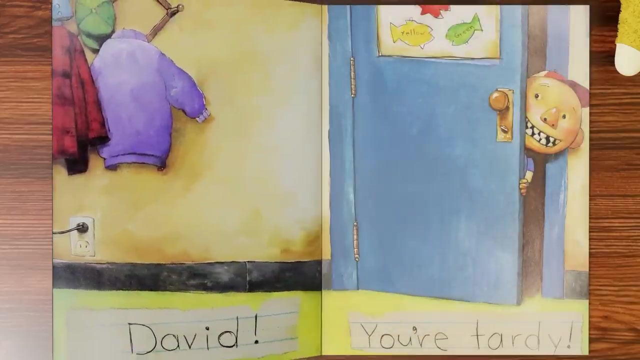 Hello and welcome back to another animated storybook by David Chanin. Next time David goes to school, David's teacher always said: No David, No yelling, No pushing, No running in the halls. Seems like the Boy of Error story is a bit later. 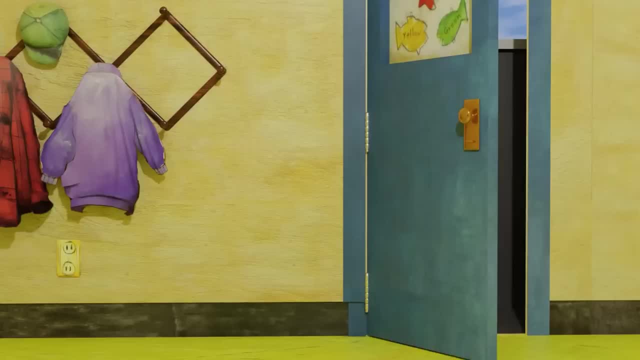 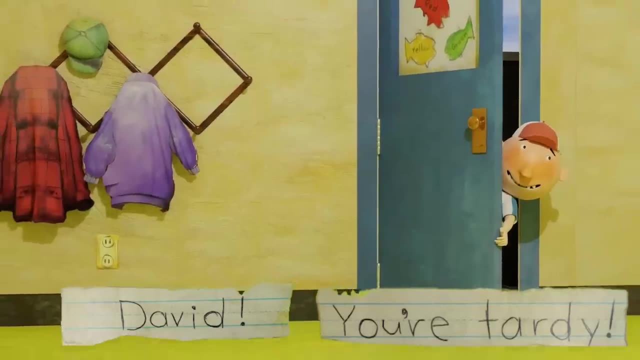 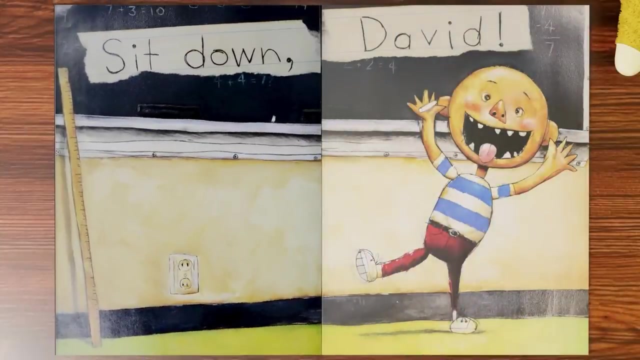 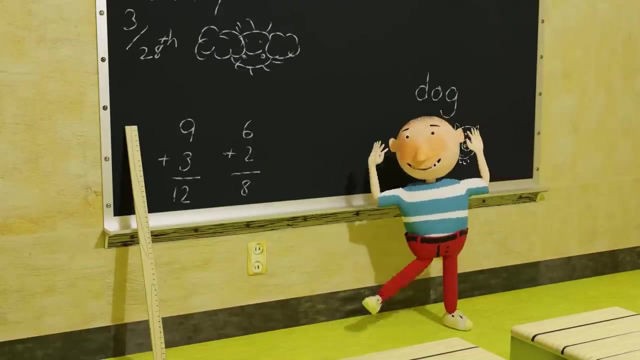 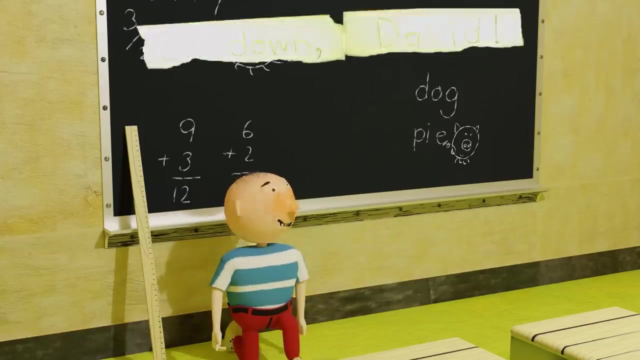 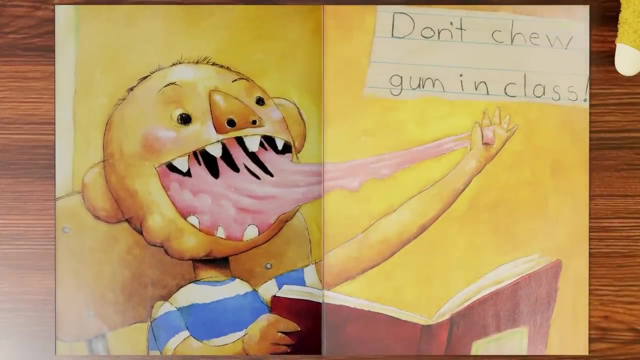 And I do remember his teacher would say: nicely, David, you're tardy. When teacher asked him to solve a problem, he would goof around show you how. And the teacher immediately said: Sit down, David. David would sometimes chew gum in class. 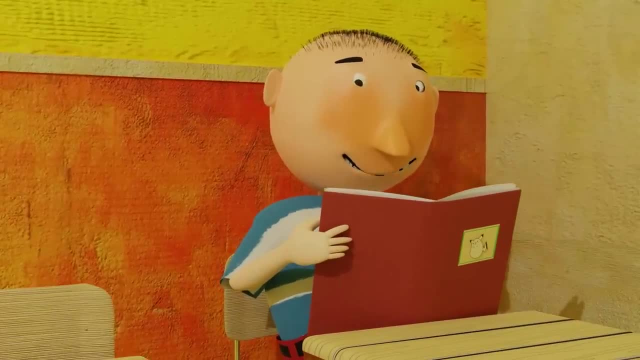 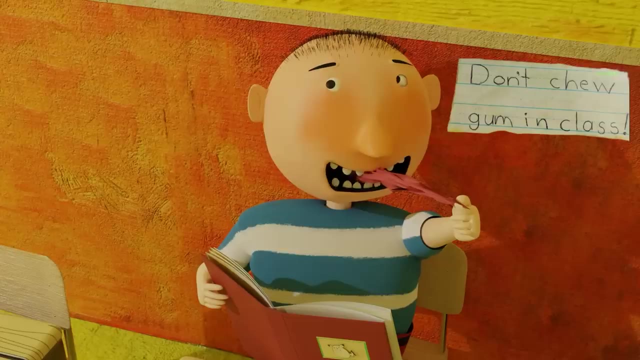 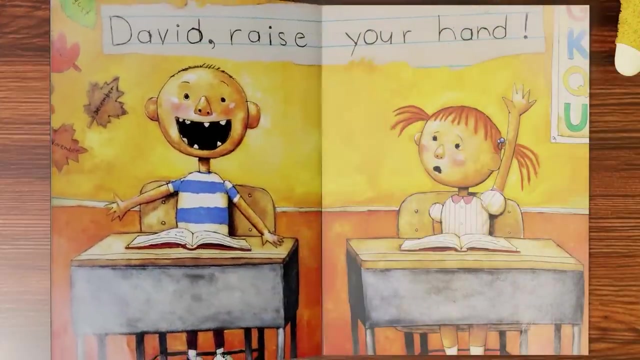 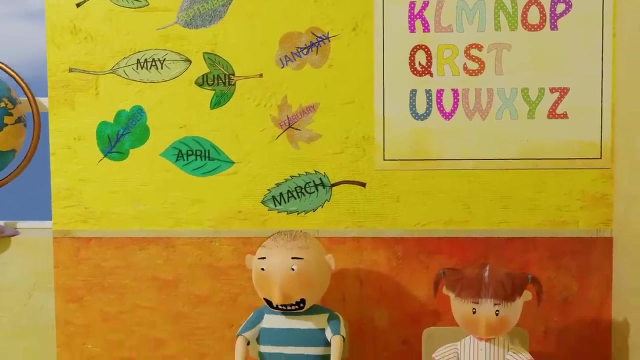 And you know chewing gum is not allowed in schools And his teacher said: Don't chew gum in class. If teacher asks you guys a question or asks students, classmates, kids a question, you guys should always raise your hand first. 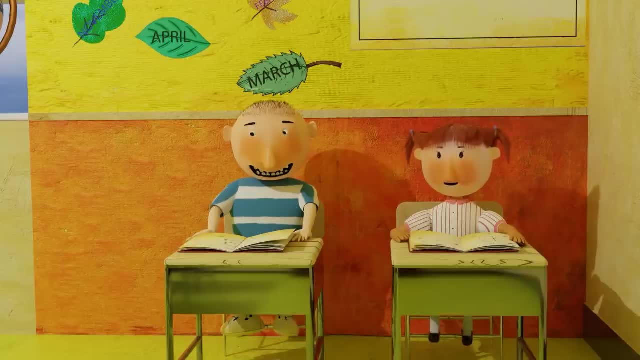 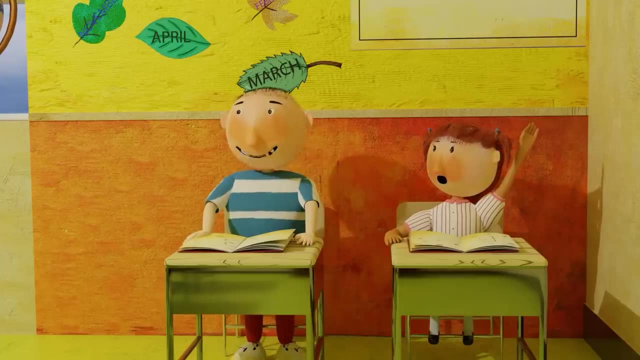 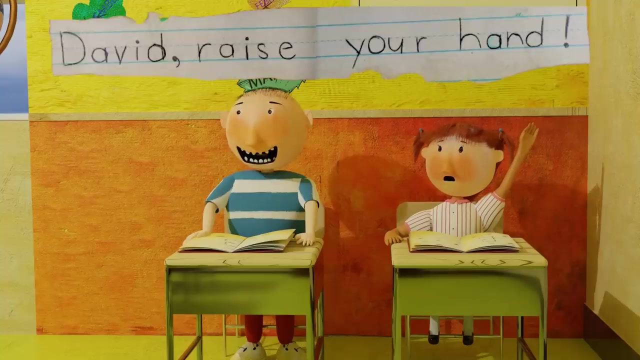 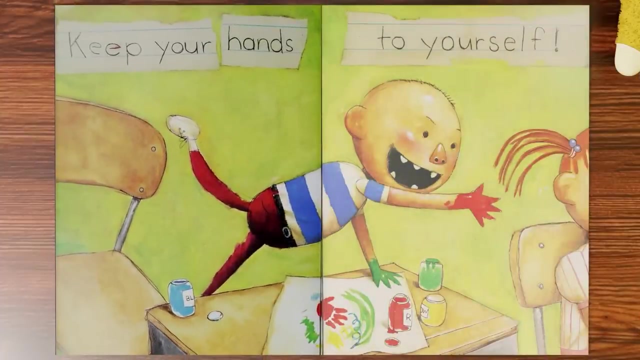 How many eyes do spiders have? In David's class, when teacher asks students a question, David would shout out the answer without raising his hand. And you know what his teacher said: David, Raise your hand. Oh, he loved finger painting. 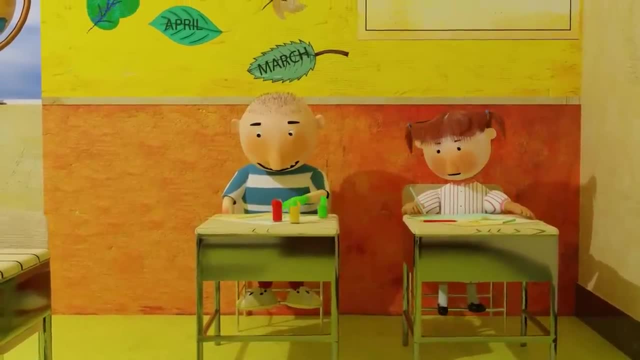 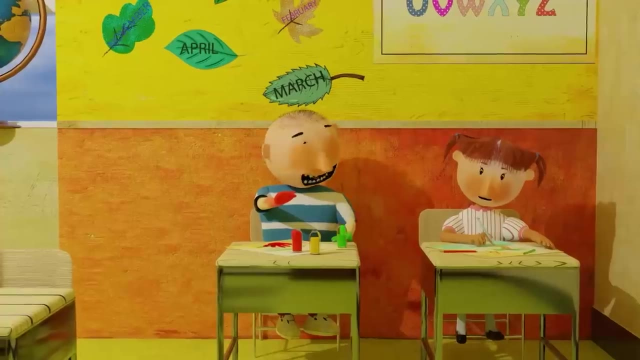 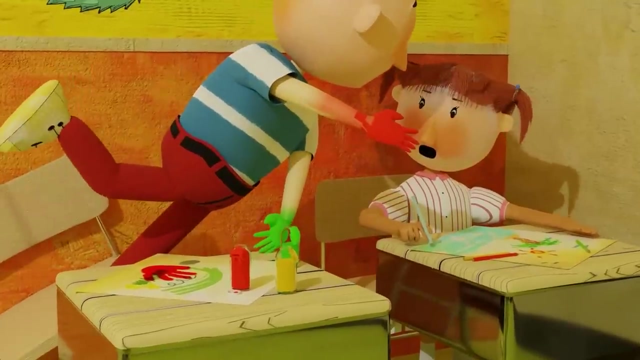 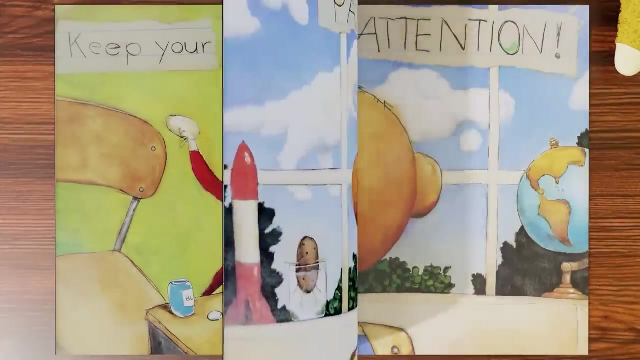 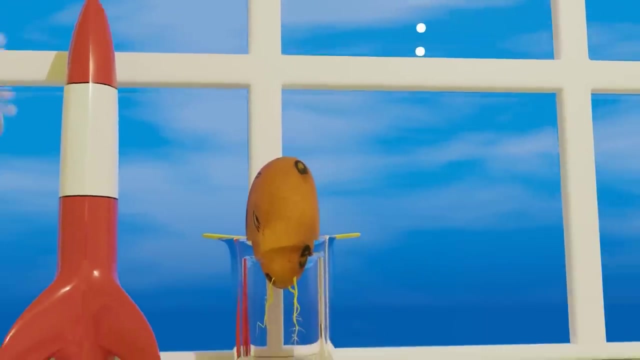 Let me tell you something funny about David. During art class, after finishing with his painting, he would love to play with paint and annoy his classmates. What teacher said coming next? Keep your hands to yourself. And sometimes he would look out the window. 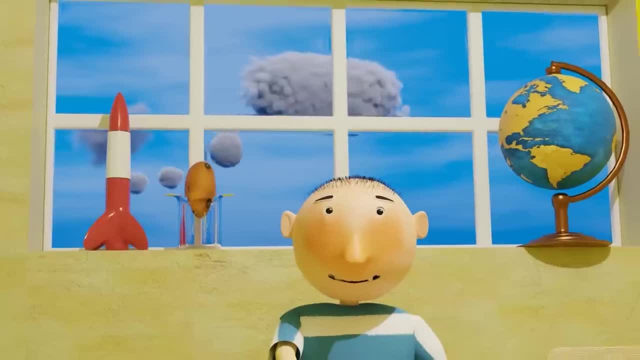 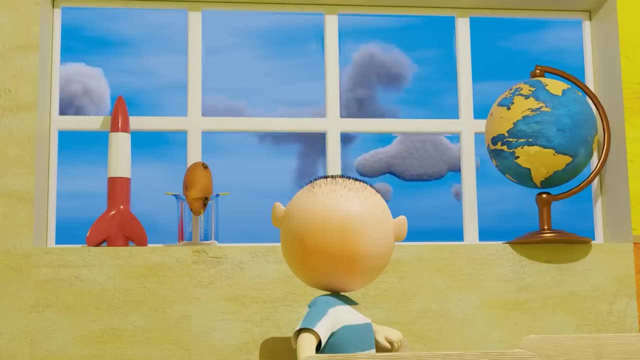 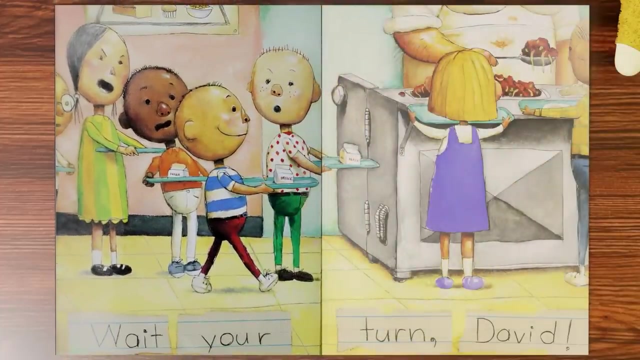 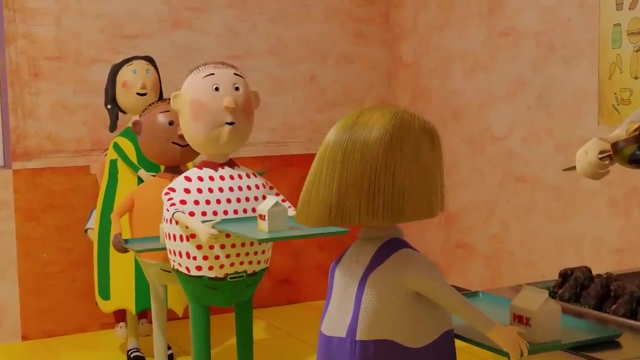 and he would dive deep in his thoughts, looking at the beautiful sky, seeing different shapes of clouds turning into different shapes like dinosaurs, cars, monsters, and until his teacher would snap him out of it. Pay attention. What David didn't like was waiting in a queue. 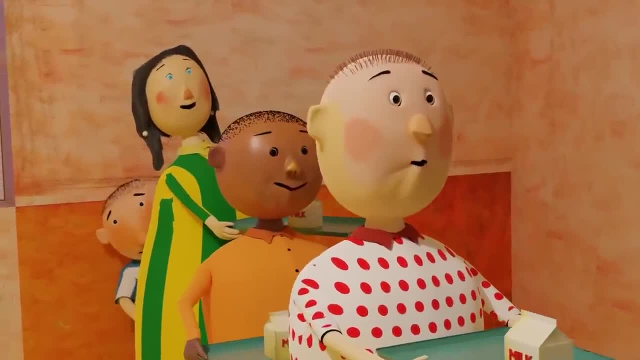 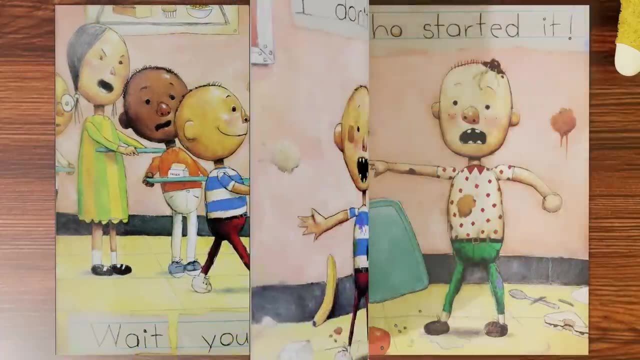 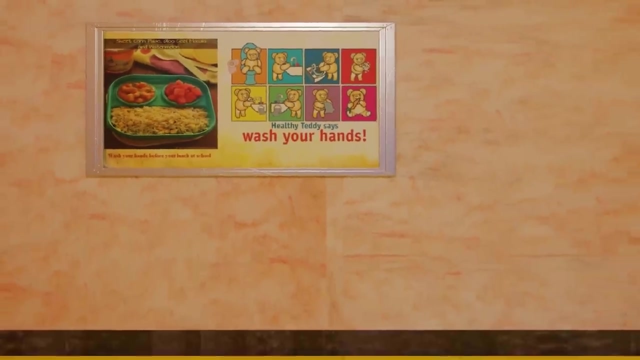 and he would like to cut in line. His teacher would say: He can't cut in. Wait your turn, David. Are you a fan of food fight? Then this particular scene is for you. You ready? He sometimes would pick food fight with his classmates. 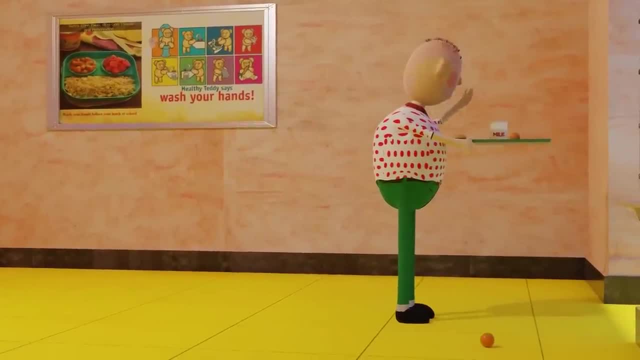 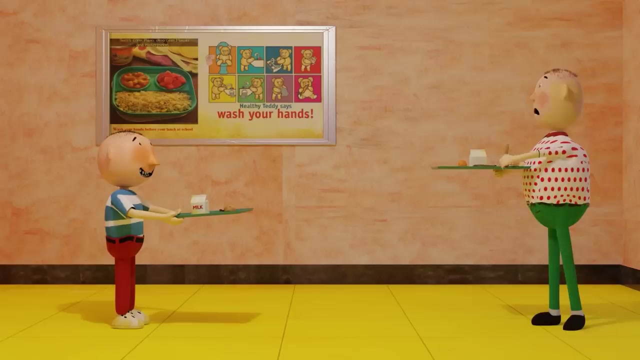 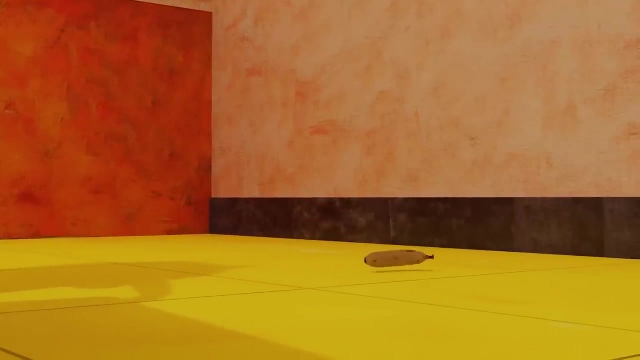 Ouch, That might hurt. What's that? Oh, smashed orange. He's laughing, Not good. He turns around. Okay, What is he going to do? He fetched a banana. That's good. Yeah, that's good. 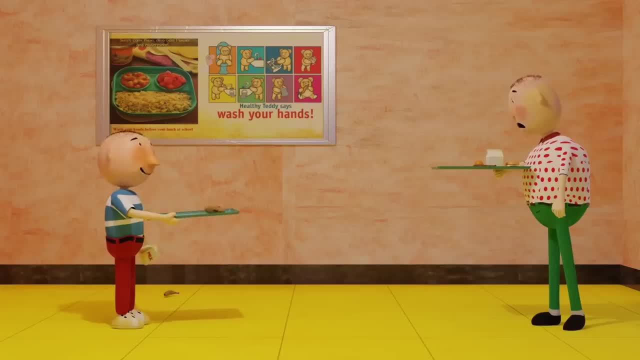 Take that Blah. So here's what happens. David's in the backseat and his teacher is using a table. He gets up and he's like, Oh crap, Where are you going? David's running after the food. 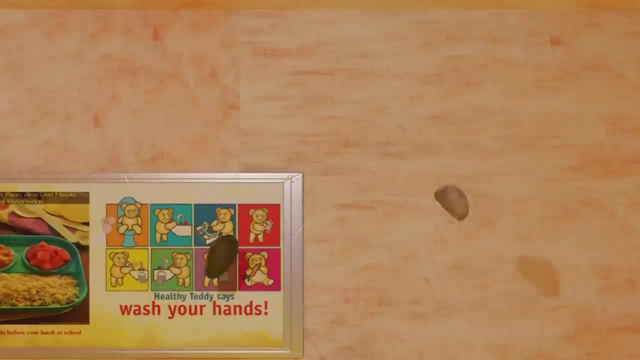 What is this? David's rushing over to the frontage? What? I can't help it. What's going on? Oh, I've got them. What's wrong with you? You can't help it, David. You can't help it. 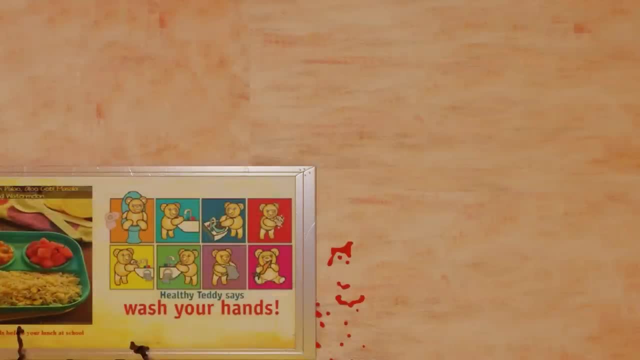 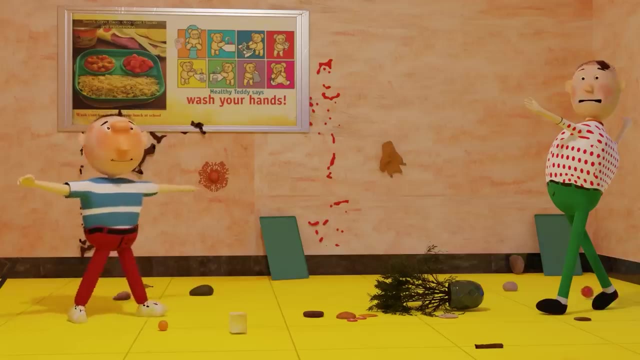 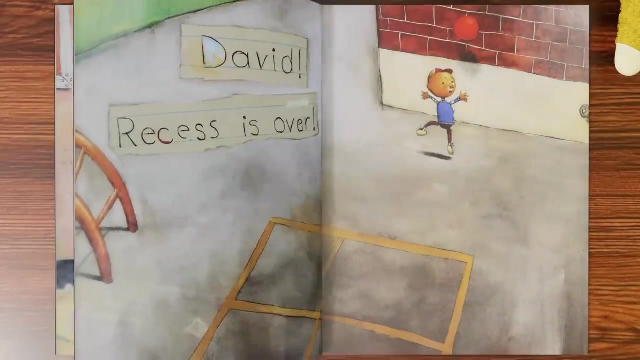 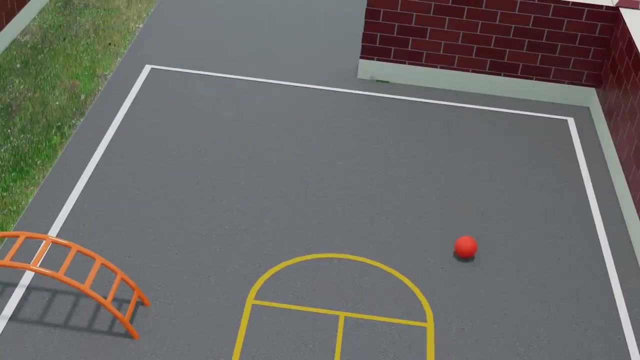 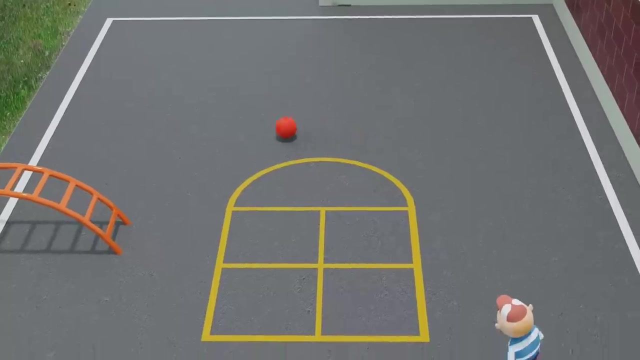 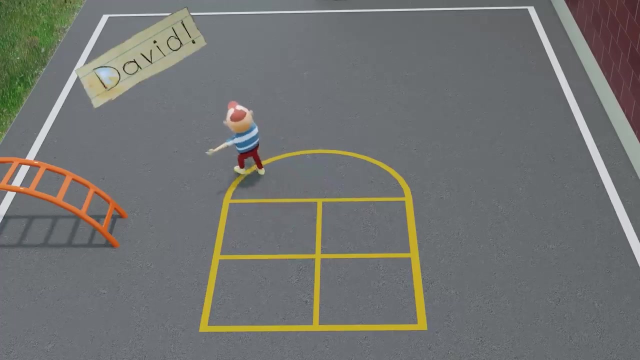 But I still have a hundred of them. Shucks, Oh my god. Who is that? Oh my God, getting too dangerous. stop it. stop it at this instance. I don't care who started it, he was still playing, the recess was over and his teachers David. recess is. 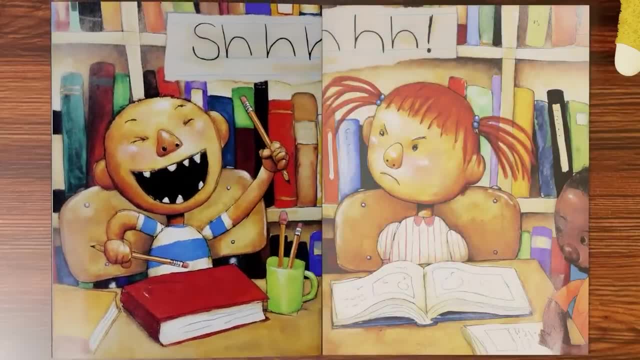 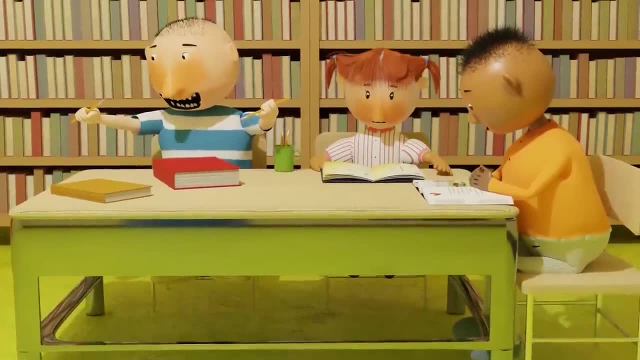 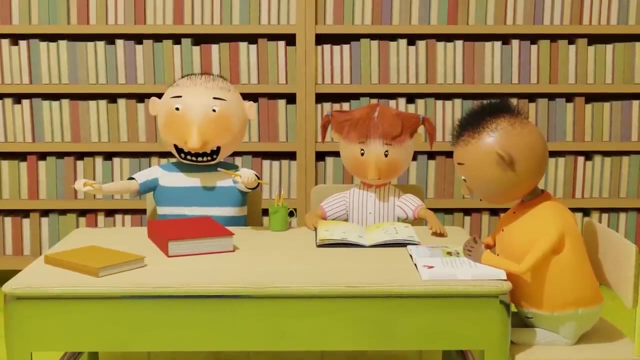 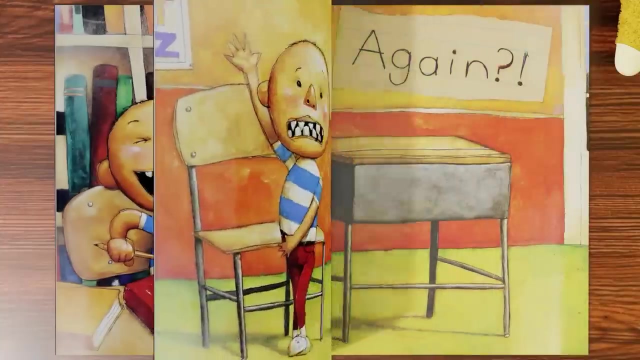 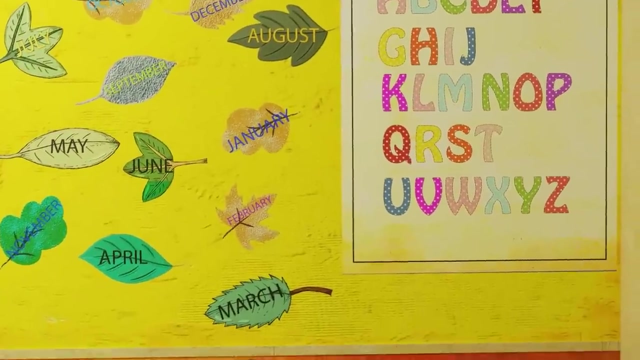 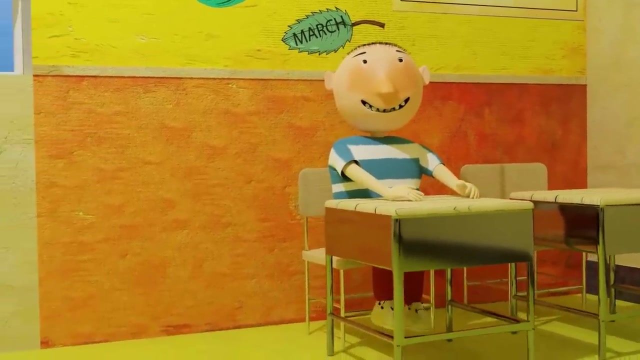 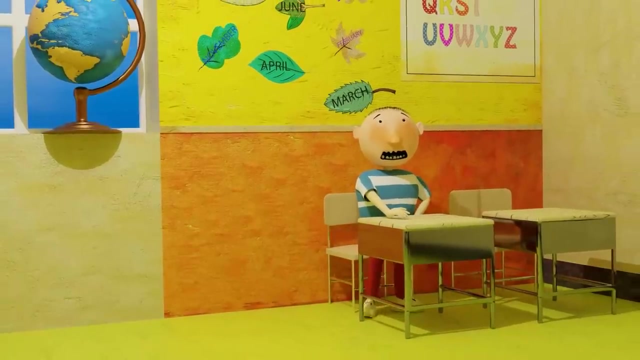 over in the library he played with his pencils, he talked loudly and his classmates Josh there, and sometimes he wanted to find a way to get out of class and he asked a permission to go to the bathroom. the best way. and David's teacher would say in a funny way: David again. 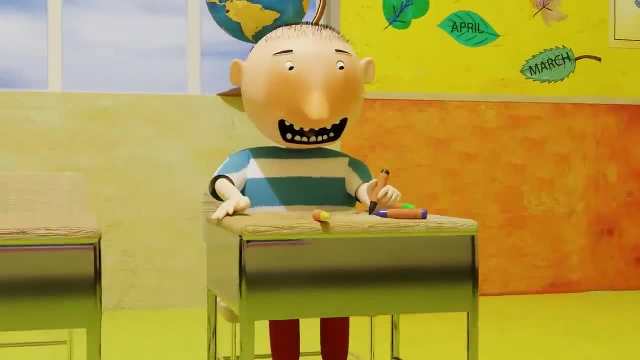 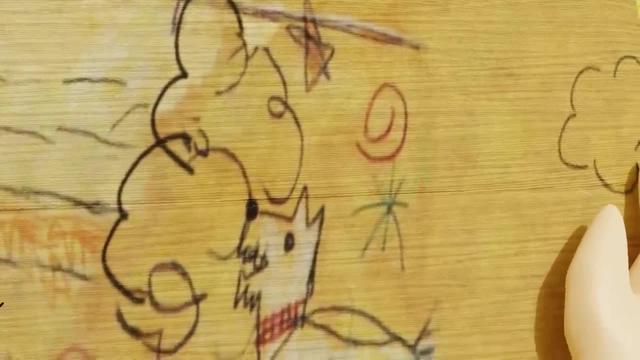 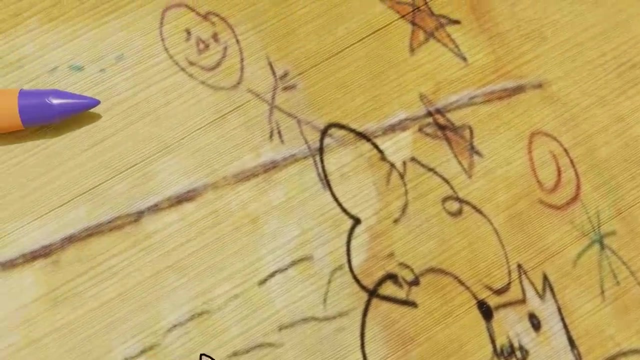 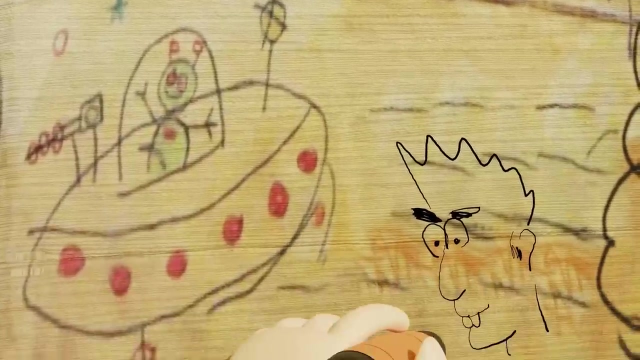 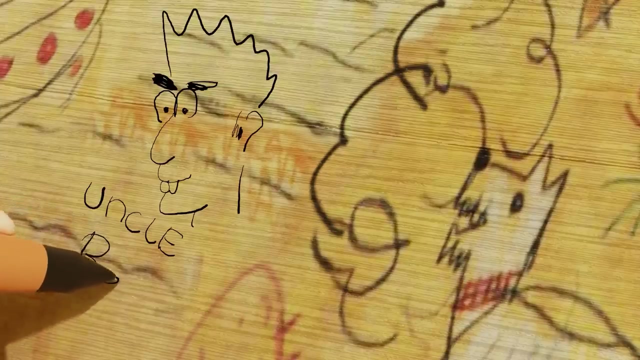 what is he doing? the last thing you want to do in your class is drawing on your desk. mm-hmm. drawings are pretty good. that's a big no, no. well, he knows how to draw my channels logo. pretty good. our drawings, David, not too bad, but not on the desk, because this may happen. 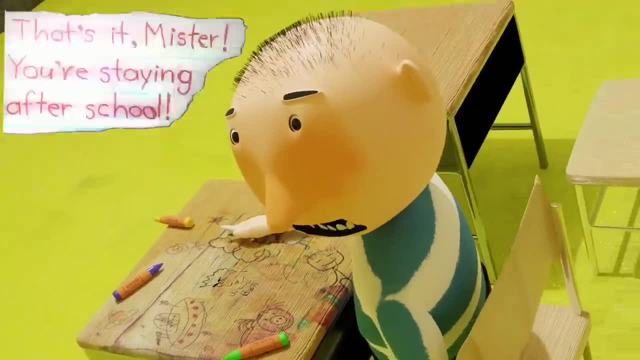 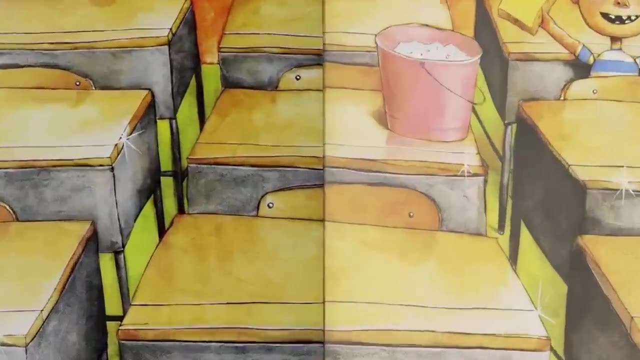 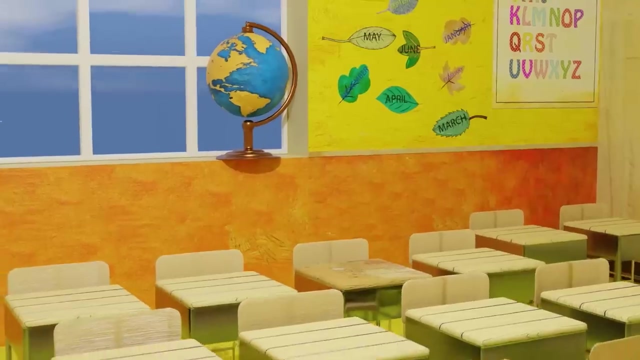 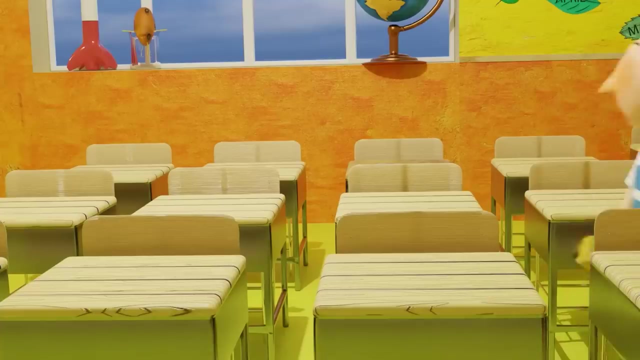 that's it, mr. you're staying after school- full- And he had to stay. And instead of cleaning one desk, he had to clean all the desks. So get to work, buddy, Get a bucket soapy water and a sponge. He did a pretty good job, David, have you?